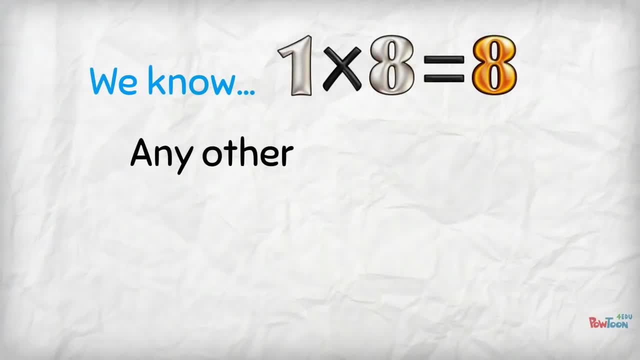 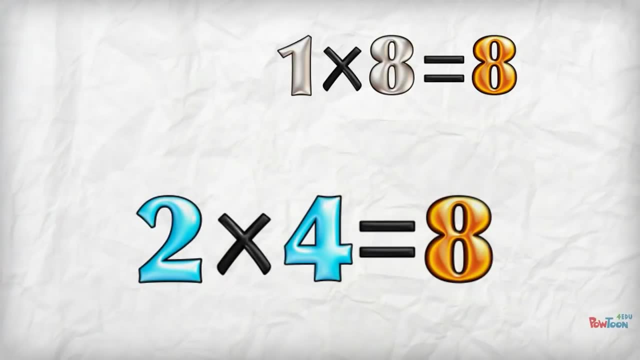 We know 1x8 is 8, But can we do it without using the factors 1 or 8?? We can use 2. 2x4 is 8. The factors of 8 are 2 and 4, as well as 1 and 8 itself. 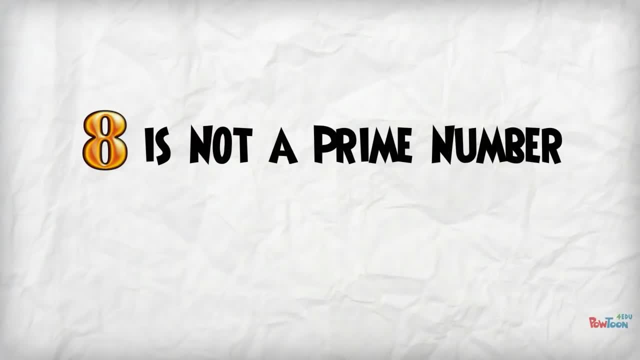 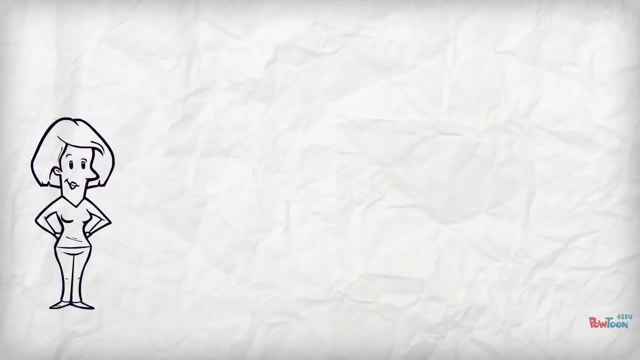 8 has more than 2 factors, So 8 cannot be a prime number. If it isn't a prime number, what is it? Have you worked it out already? This program is about prime numbers and composite numbers. If a whole number greater than 1 is not prime, 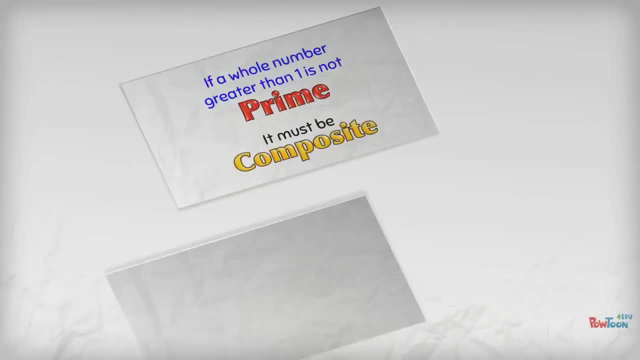 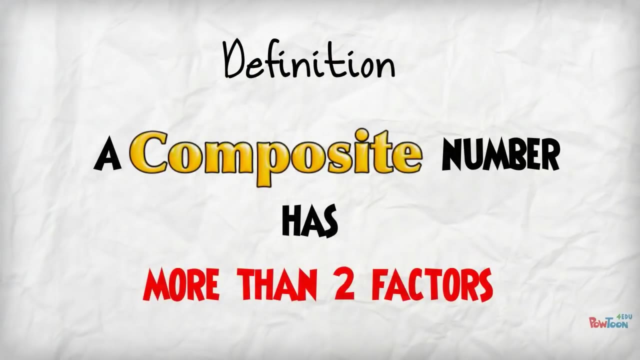 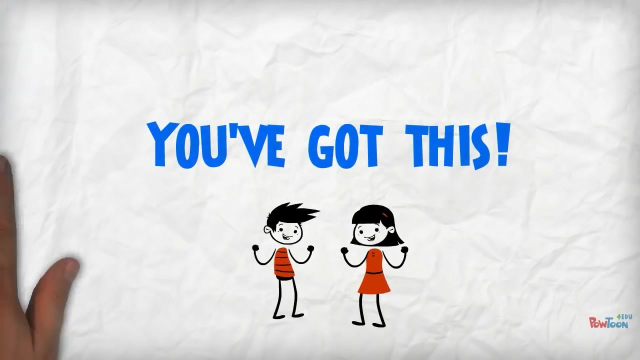 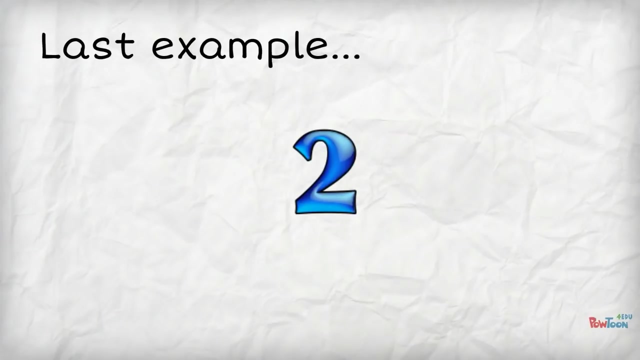 then it must be composite. Let's give it a definition. A composite number has more than 2 factors, like we just saw with our example of 8. I think you've got this. My last example is a very special number: 2, The first even number. Is it prime or composite? 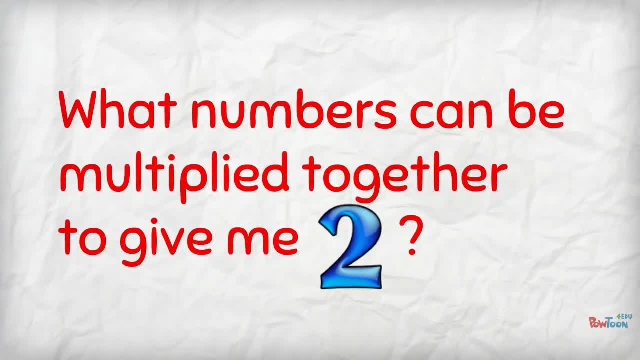 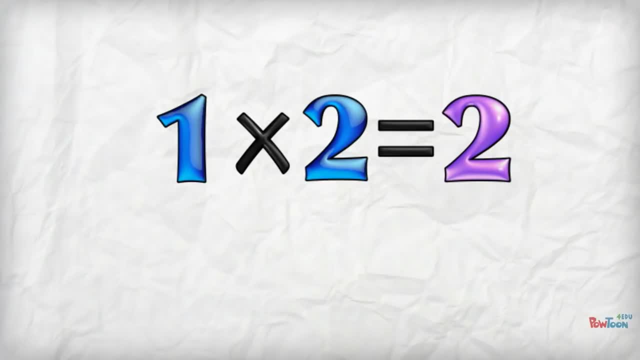 Say to yourself What numbers can be multiplied together to give me 2? 1x2 is 2 or 2x1 is 2? There is no other way to multiply up to 2. 2 has 2 factors, 1 and 2 itself. 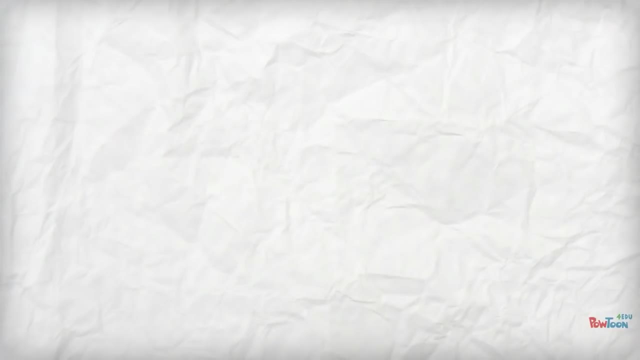 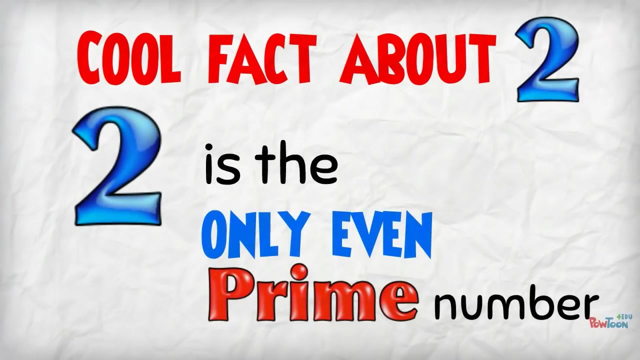 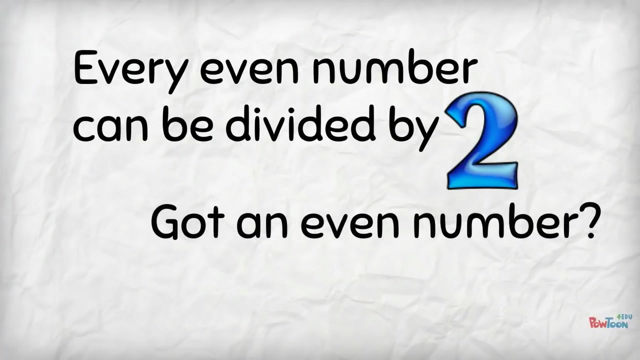 So that means 2 is a prime number. The cool fact I want you to get about 2 is that 2 is the only even prime number. Every even number can be divided by 2, So anytime you are given an even number, you can always say that 2 is going to be one of the factors. 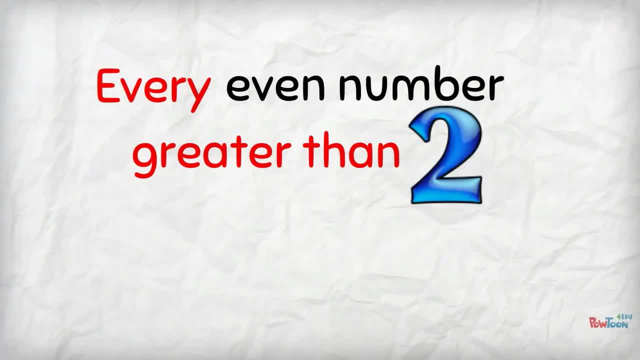 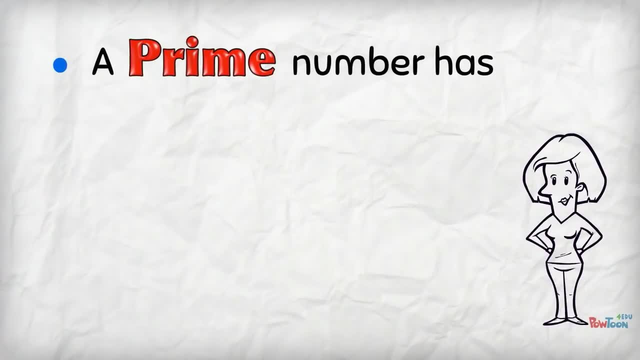 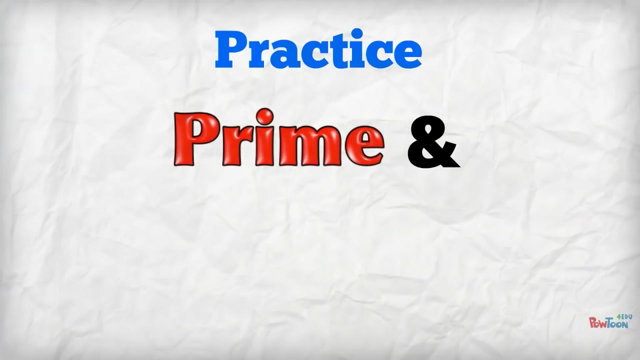 And that means Every even number higher than 2 is always a composite number. Remember, A prime number has exactly 2 factors, 1 and the number itself, And a composite number has more than 2 factors. Now it's your turn to practice with prime and composite numbers. 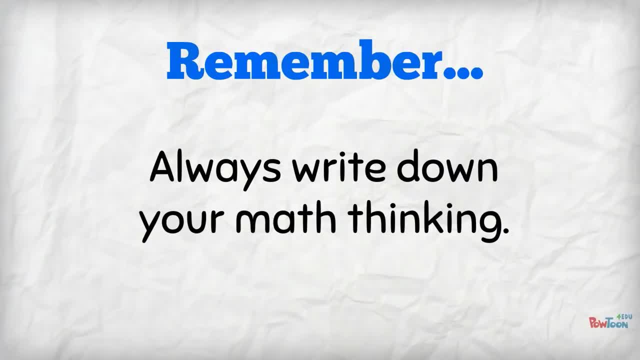 Remember to prove your answer by showing your math thinking, just like I did, Exploring Prime and Composite Numbers.